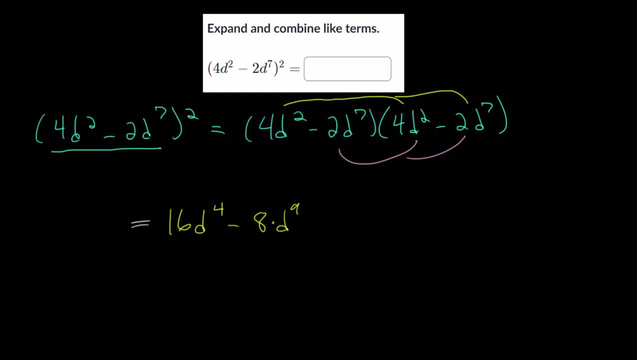 And then we start over with the minus 2d to the seventh. We're going to multiply that to 4d squared, And minus 2 and 4 gives us minus 8.. d to the seventh times d squared is d to the ninth. Notice. 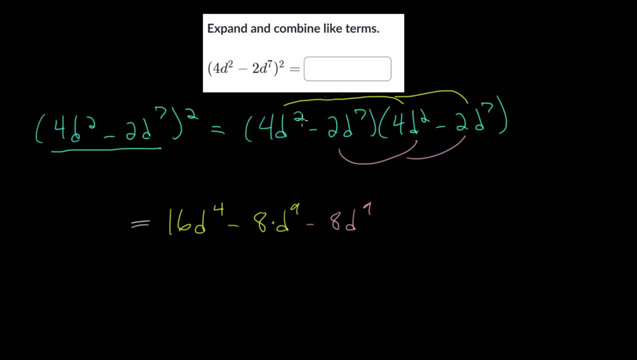 we got the same term twice. And then we take our minus 2d to the seventh and multiply it by minus 2d to the seventh, And minus 2 times minus 2, that's positive 4.. And d to the seventh times d. 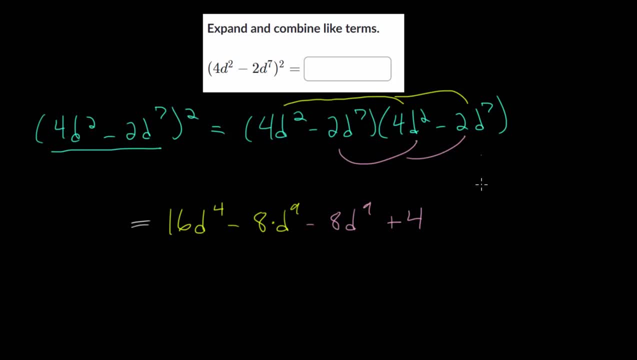 to the seventh. Well, we have seven here and we're multiplying d another seven times. So in total that is 14.. So we have 16 d's multiplied together. And we can simplify, We can combine these two middle terms. since they are like terms. They both have a d to the ninth in them. So we have 16 d to the fourth. 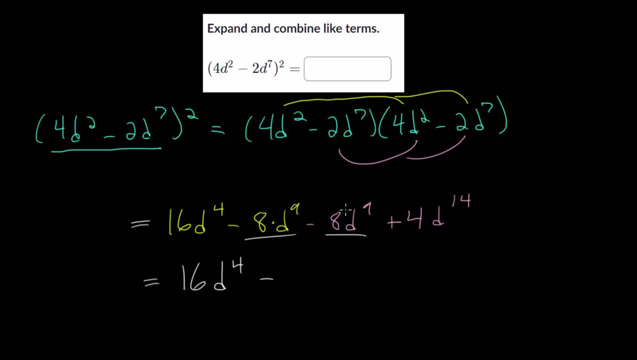 Now we're subtracting 8 of this thing, And then we're taking away 8 more of that same thing, And so we in total are taking away 16 of the d to the ninth And we have plus 4 d to the 14th. So this: 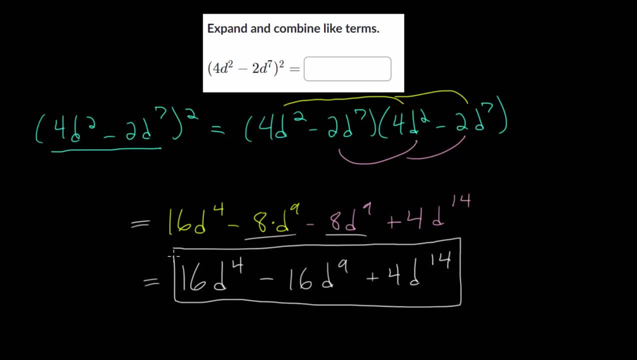 should be our final answer, And the way to check this is to use the formula. So remember the formula a plus b squared, which we looked at in the intro video, is just a squared plus 2ab plus b squared, And we would just need 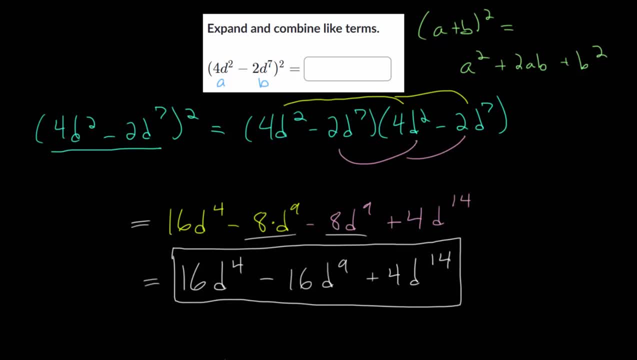 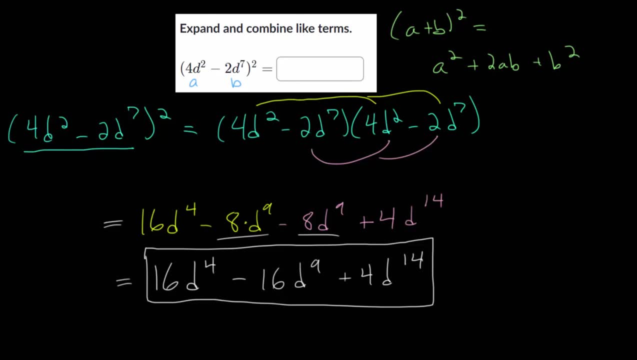 to identify what a and b are. So let's quickly do this, just so that we can feel certain that we're doing this correctly. So for us, this in: we have a squared, so that's 4d squared, and we're squaring that and then plus 2 times a. 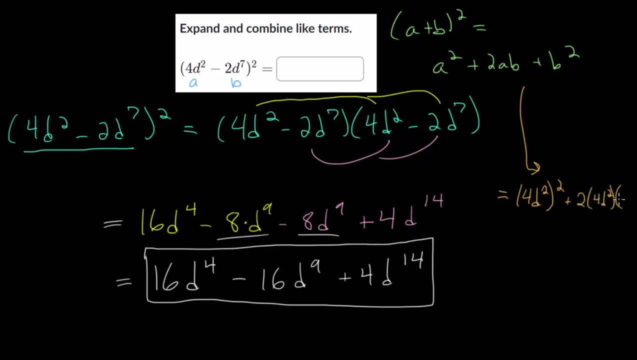 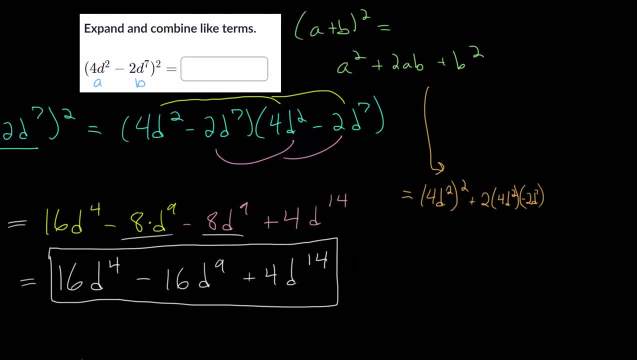 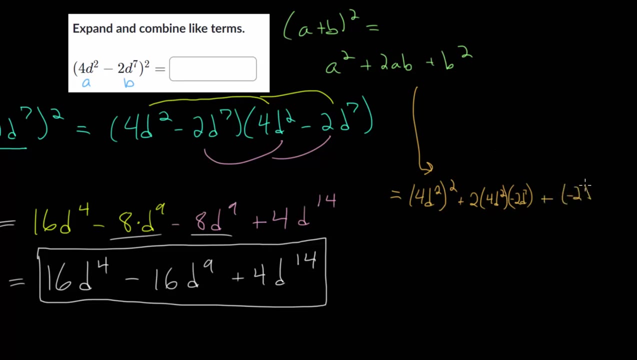 so 4d squared times b, which is minus 2d to the seventh- and let me just make actually a little bit more room so we can keep writing this- and then we have plus b squared, and so b, we know, is minus 2d to the seventh. and so now we just simplify, so, squaring this, we get 16d to the fourth. we can. 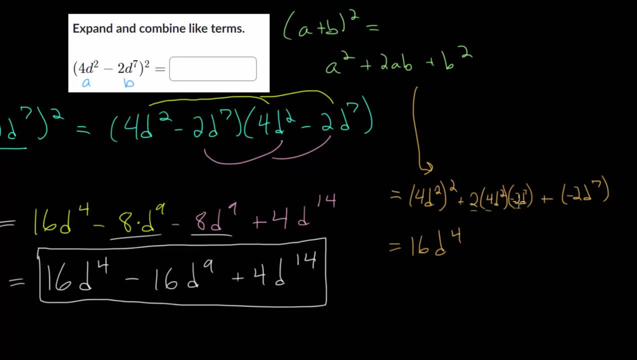 multiply all the number terms here, so that's 8 times minus 2, that's minus 16d. squared times d to the seventh is d to the ninth, and then we have minus 2d to the seventh and we're squaring this. so minus 2 times minus 2, that's positive 4d to the seventh. 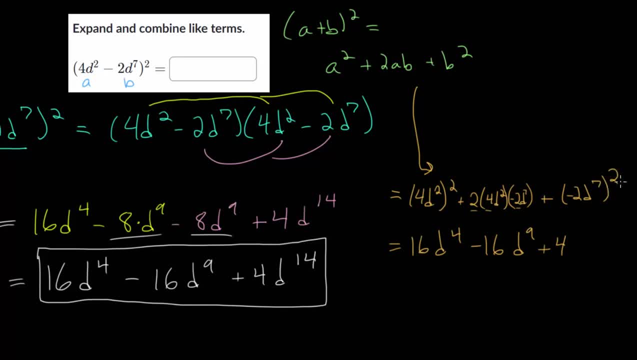 so we have an exponent to an exponent. so we multiply that, so we get 7 times 2, which is 14.. and notice: 16d to the 4th, minus 16d to the 9th, plus 4d to the 14th, we have the exact same answer. 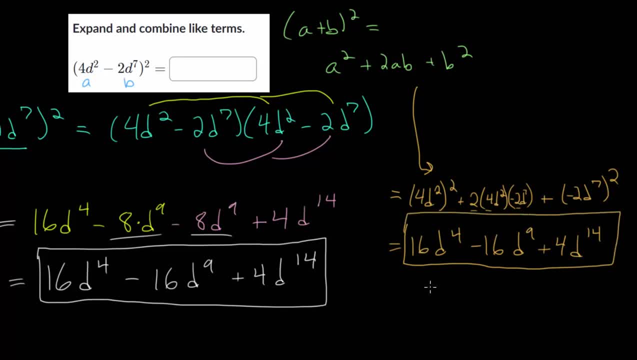 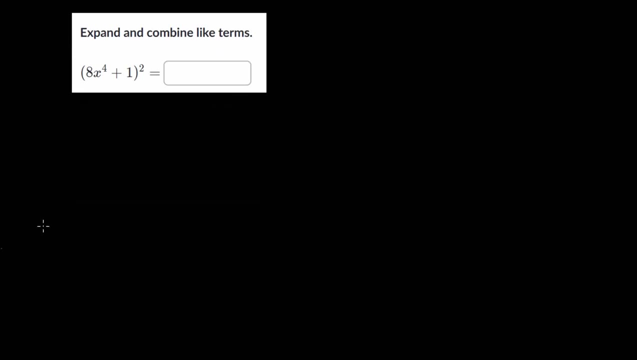 using the formula, and since we arrived at the same answer using two different methods, we can feel confident that we are doing this correctly. so this will be our final answer here, and let's just do one more problem, and for this one again, we'll just use the distribution method and i. 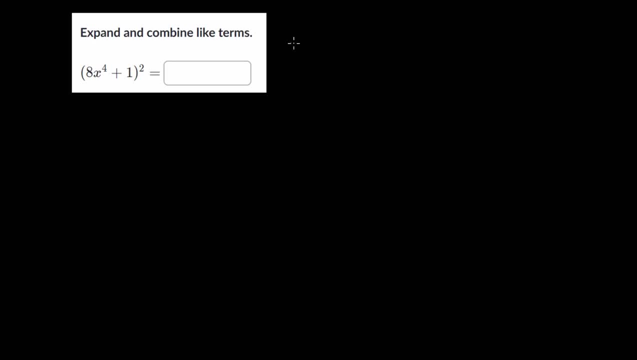 encourage you to check this problem on your own using the formula. so let's just rewrite 8x to the 4th plus 1. we need to rewrite it twice, since we are squaring it. so we have 8x to the 4th plus 1. 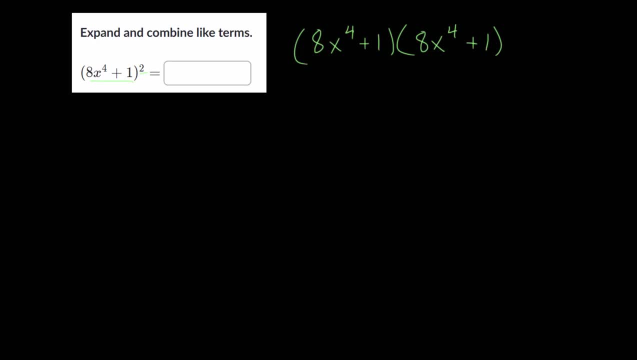 times 8x to the 4th plus 1.. and now we will distribute the 8x to the 4th to both of those terms and we will also distribute the 1 to both of those terms. so 8x to the 4th times 8x to the 4th. 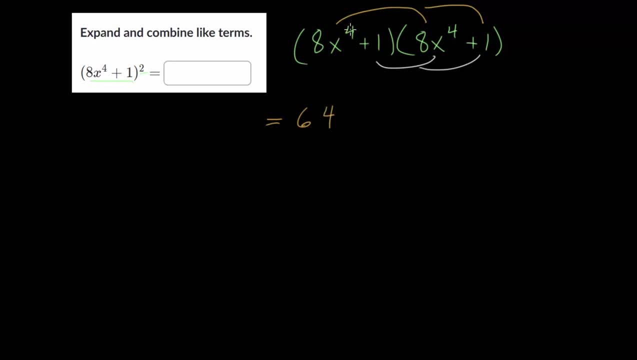 8 times 8 is 64, and we have 4 x's here and 4 more here. so in total we are multiplying 8 of them together, and then 8x to the 4th times 1. that's just positive 8x to the 4th, and then we do 1. 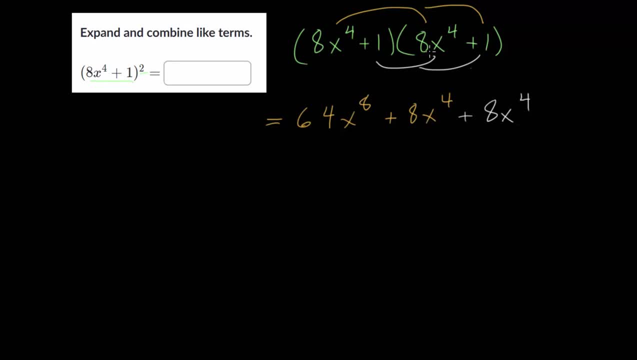 times 8x to the 4th, which again is just 8x to the 4th, and then 1 times 1 is just 1, so we get plus 1 at the end, and now we just need to simplify everything. so notice that we have like terms here. we have 8 of these x to the fourths and we're 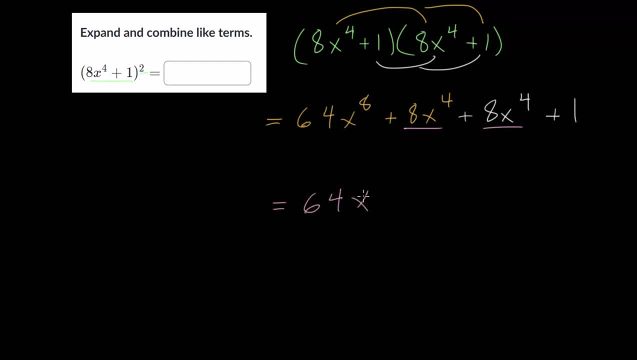 adding 8 more x to the fourths. so that's going to give us 16 of those x to the fourths and we still have the 64 x to the 8th and the plus 1.. so this should be our final answer, but